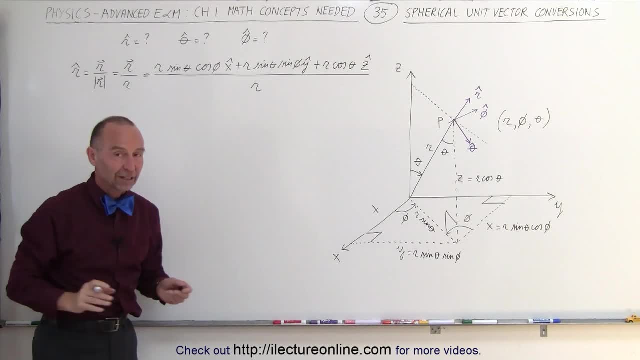 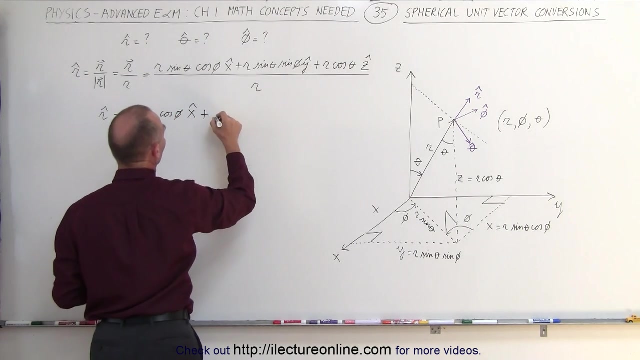 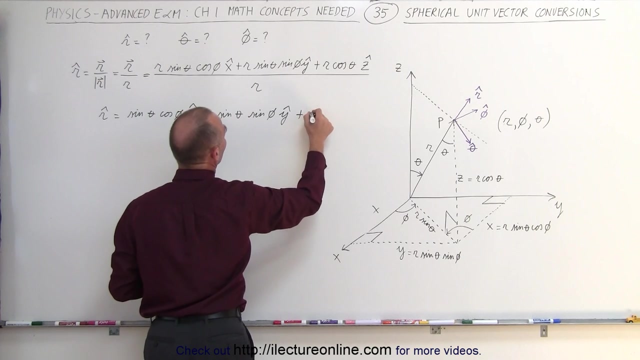 divide it by r. That's the magnitude of the r vector, the position vector, which then cancels out all the r's. In other words, the r unit vector can be written as: the sine of theta cosine of phi in the x direction plus the sine of theta times the sine of phi in the y direction plus 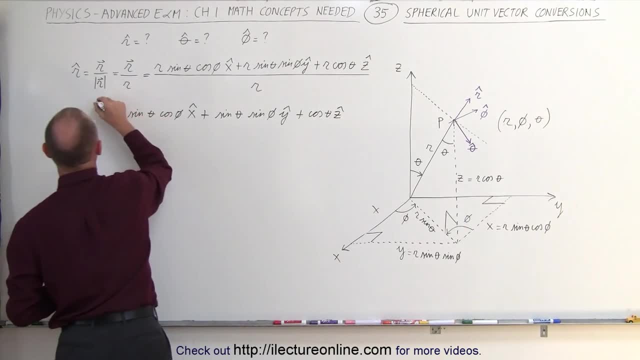 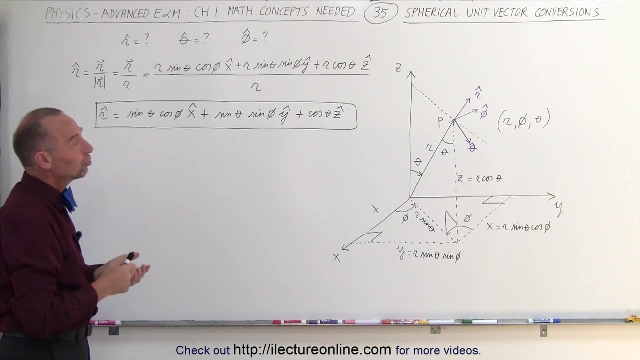 the cosine of theta in the z direction. We tienen r unit vector, unit vector expressed in terms of the x, y and z unit vectors. we should be able to do a similar thing for the theta unit vector and for the phi unit vector. let's go ahead and try to do that. 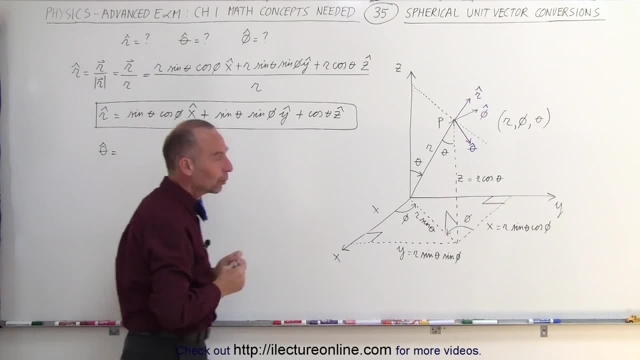 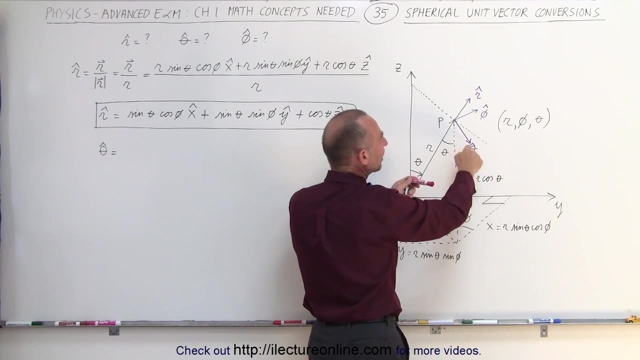 theta unit vector can be described as follows. well, we're going to do the easy one. first, notice that the phi unit vector is right. here i should say theta unit vector. this is theta. notice that if i bring the point p all the way to the z axis, then the theta unit vector would stick straight. 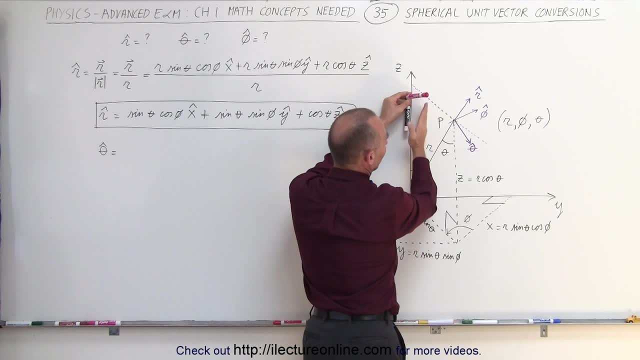 out and there would not be any z component as we start dropping this r vector down to the x, y plane. notice: at this point the theta unit vector would only point, it would point completely into the negative z direction right here. so you can see that the z component simply depends on the angle. 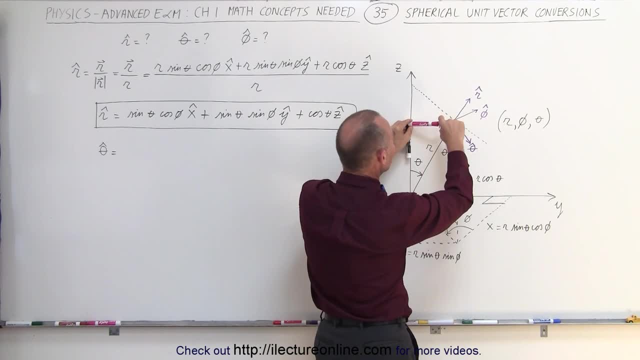 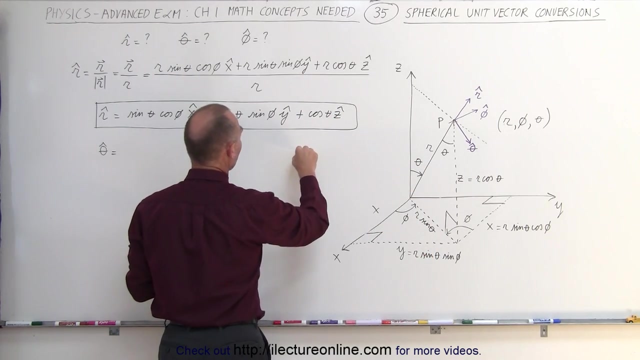 theta. if the angle theta is zero, then the z component is zero. if the angle theta is 90 degrees, then the z component would be a negative in the negative direction. that's loss. that sounds like a negative sign of the angle theta. so we can write the z component as the minus sine of theta in the z. 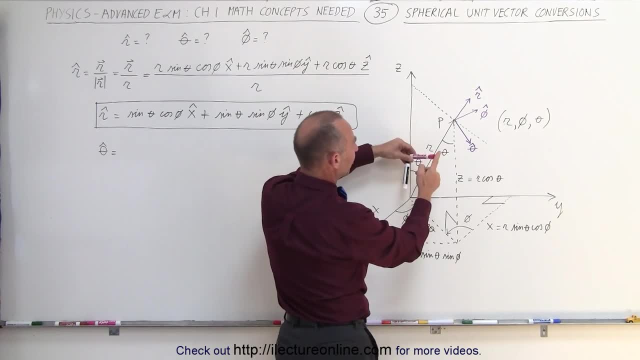 direction. again like here: there's my theta unit vector. when p is at the z axis, my unit vector looks like this: when the angle theta increases- notice: when it becomes 90 degrees the z component is a maximum, the code, the sine of 9 degrees is 1. so therefore we use a sine of theta and it's negative because when the 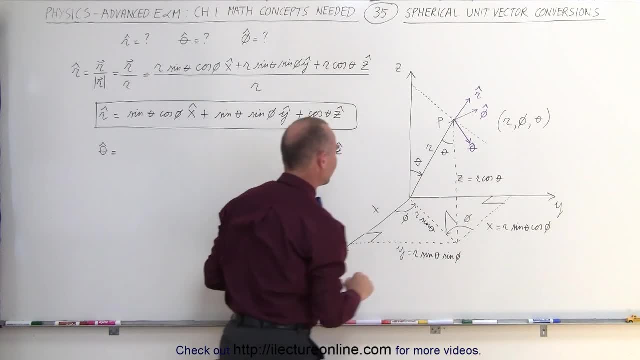 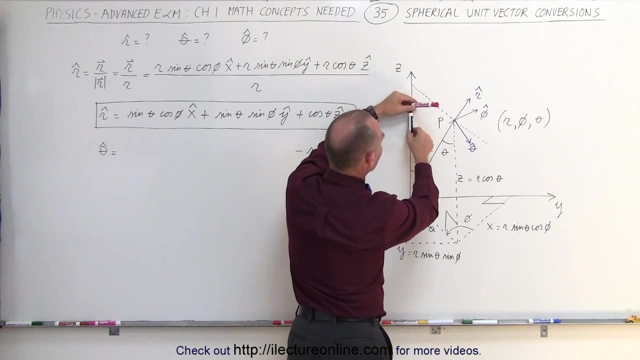 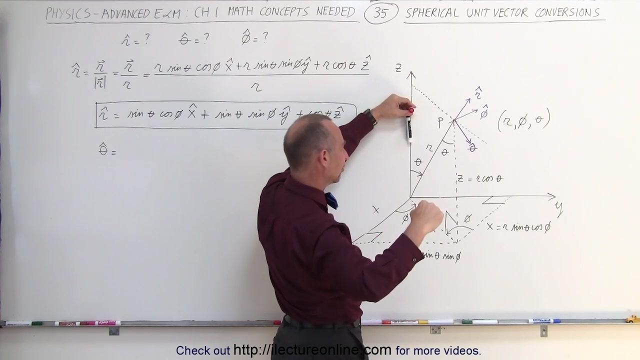 angle is 90 degrees, it's pointing in the negative z direction. what about the x and the y directions? let's see here. notice that if i have my unit vector like this, here's my angle. phi. notice that the x-axis is straight out of the z-axis and the z-axis is pointing in the negative z-direction. so 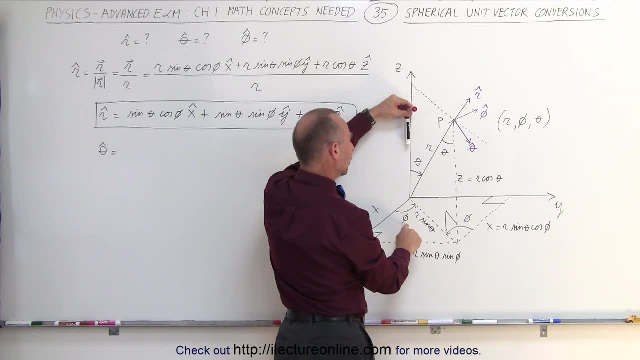 if i make my z-axis zero, then i can see that my z-axis is pointing out of the z-axis. that's what i'm looking for. so if i make my z-axis zero, then i can see that my theta unit vectors pointing straight out like this, which means it depends on the phi angle in terms of when phi is. 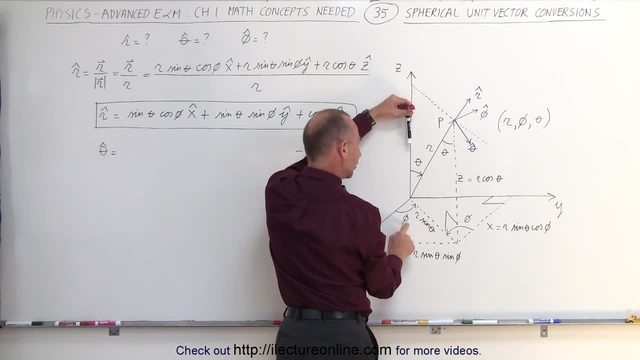 zero, then i have a maximum magnitude in the x direction. when phi is equal to zero and when phi is equal to 90 degrees- notice- my theta unit vector points in this direction and there's no x component it at all. so, based upon the phi, the phi angle, it is maximum, the angle is zero and zero when the 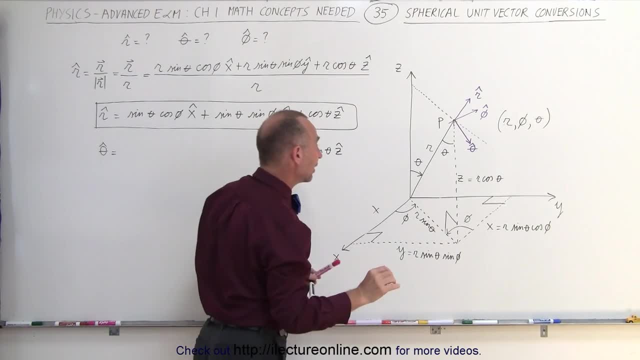 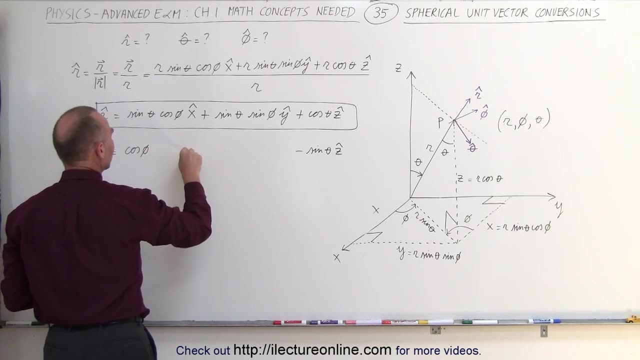 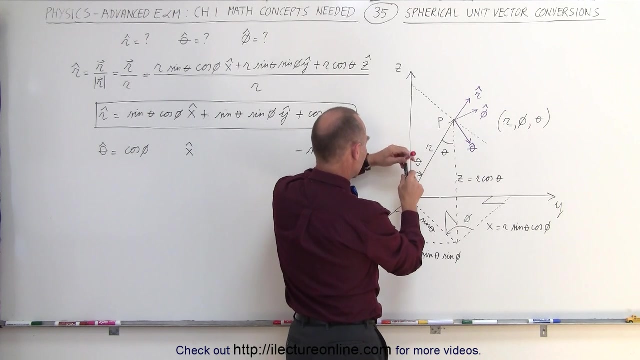 angle is 90 degrees, which means that it depends on that angle via the cosine. in other words, it is equal to the cosine of phi times the x unit vector. now, how does it depend on the theta vector? all right, so when theta is equal to zero, zero degrees? so when phi is equal to zero degrees? 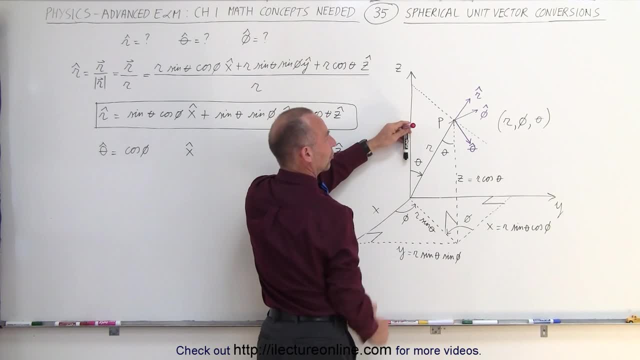 and theta is equal to zero degrees. notice that the theta unit vector sticks straight out. when theta becomes equal to 90 degrees, that means the theta unit vector is straight down and then there's no component relative in the x direction. so that means it also depends on theta in terms. 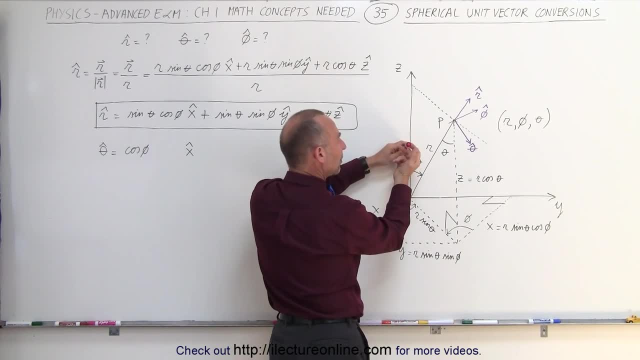 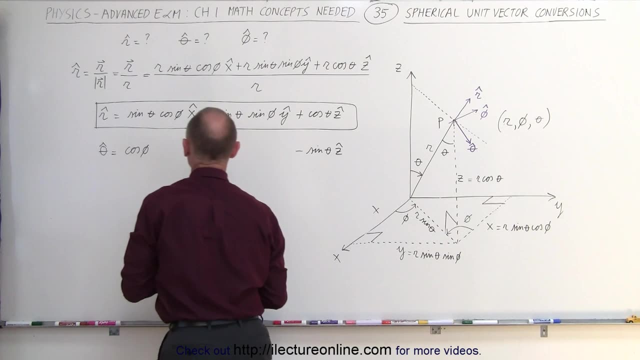 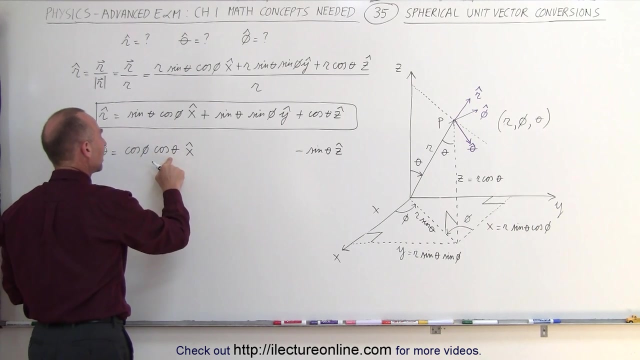 of cosine. when theta is equal to zero, we have a maximum x direction. when theta is equal to 90 degrees, we have zero in the x direction, which means it also depends upon the theta angle in terms of the cosine. so we have the cosine of phi times the cosine of theta times the x component. that would 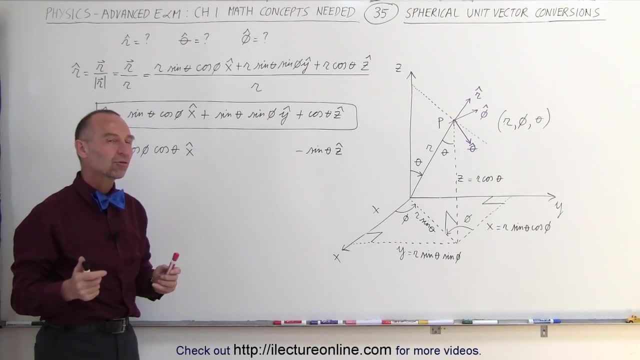 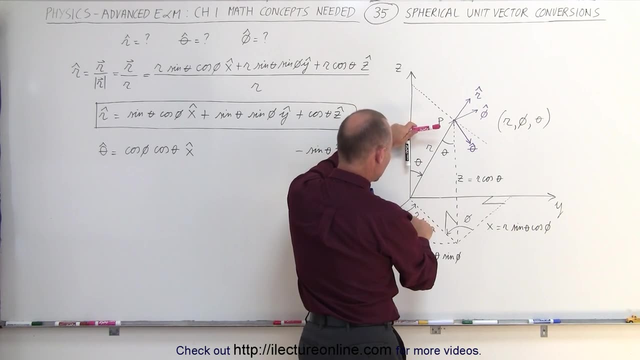 then be the x component of the theta unit vector. now let's try to figure out for the in the y direction. first of all, you can see here that if the angle you phi is 90 degrees, the unit vector, theta unit vector, points into into the y direction when the 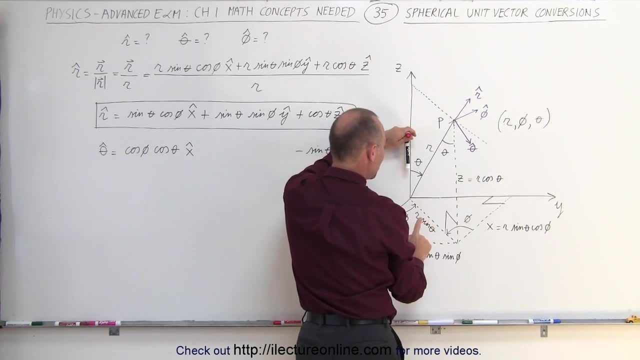 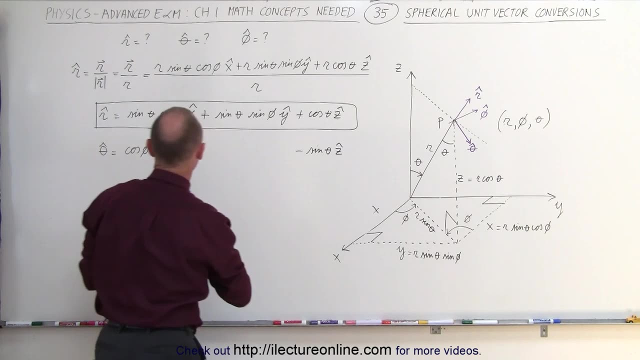 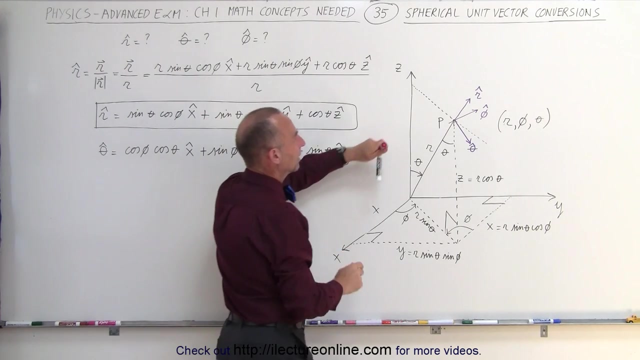 angle is zero degrees, it does not point in the y direction at all, which means that at zero degrees, at zero, at nine degrees at once. so we use the sine related to the phi angle, so that would be equal to plus the sine of phi. what about the theta angle? again, when the angle is zero, when the point p is. 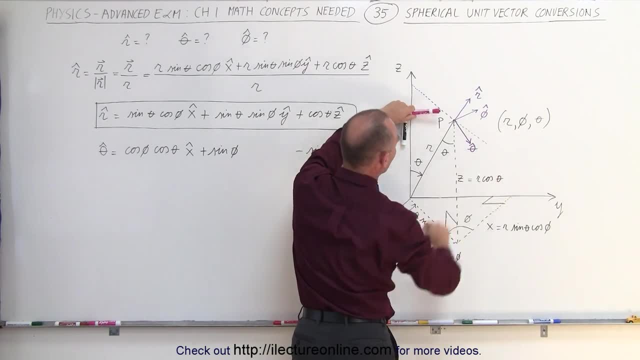 directly on the z axis, we have the sine of phi and we have the sine of phi and we have the sine of phi. and so, as you can see, on the x axis- notice- we have a maximum direction in the y direction. when the angle is 90 degrees, we have zero direction in the y direction, which means that that component in the 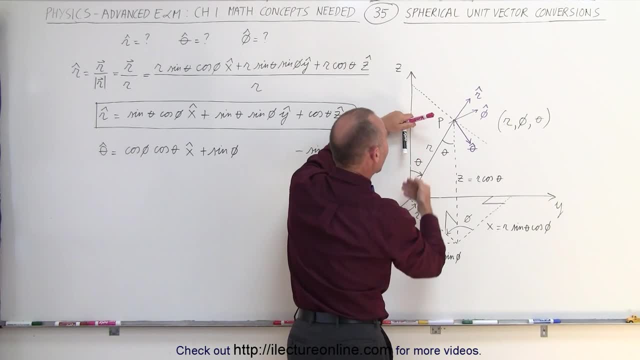 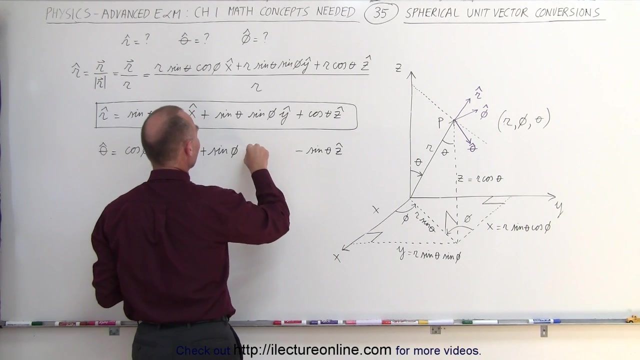 y direction depends on the angle theta in terms of the sine. zero or is the cosine? let me think about that again. if it's zero degrees, we get a maximum direction. when it's nine degrees, we get zero. that's the cosine. so depends upon the angle theta via the cosine. so there's the cosine of theta. 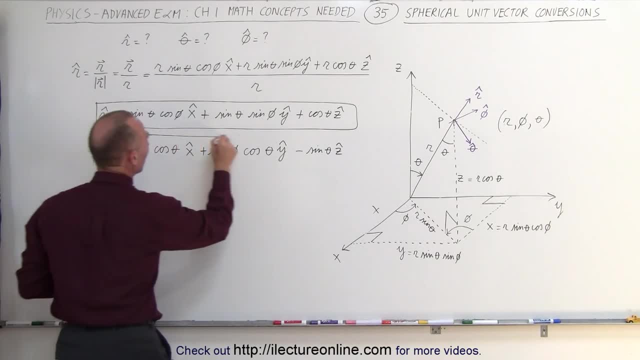 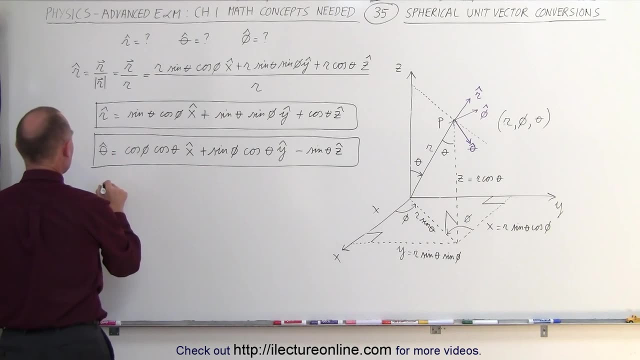 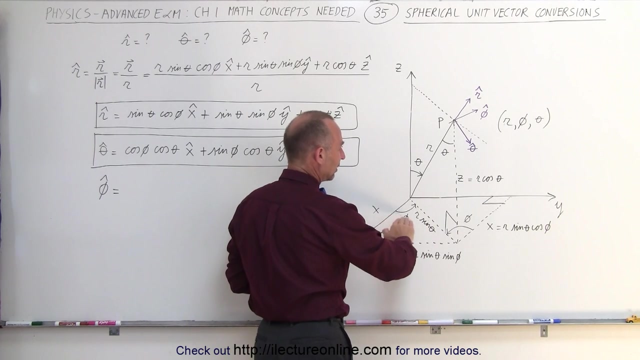 in the y direction. so now we have a relationship between the theta unit vector and x, y and z. finally, now we need a relationship between the phi unit vector and x and y and z. well, first of all, the with the with the phi unit vector right here, since the phi unit vector is in the xy plane. 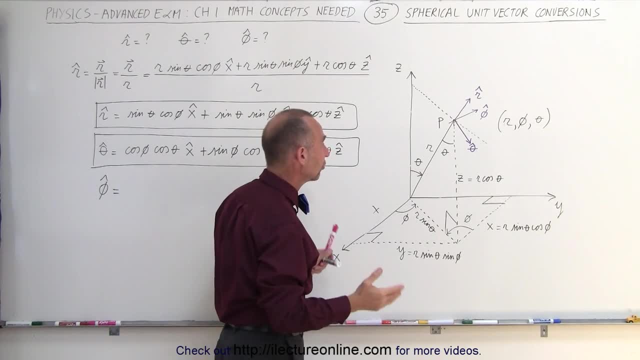 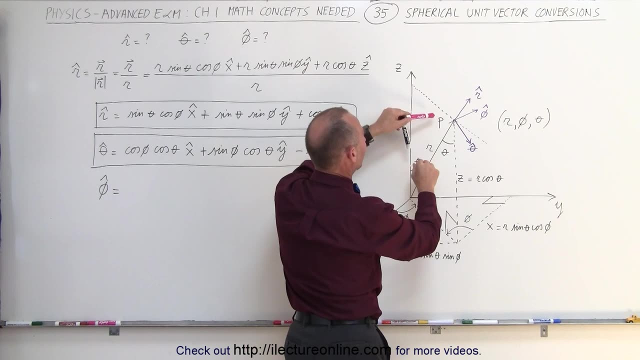 there's no z component at all, so the z component is equal to zero. now in the let's see here: so we have the phi unit vector, which is like this: when, when we are- okay, let me try it this way- so when the angle phi is equal to zero. 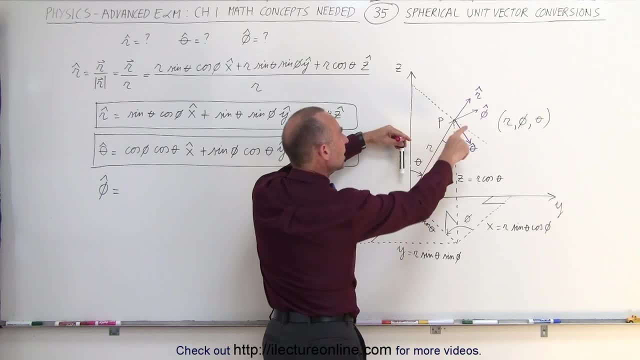 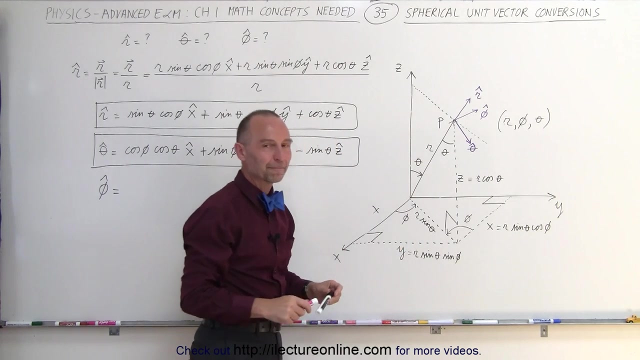 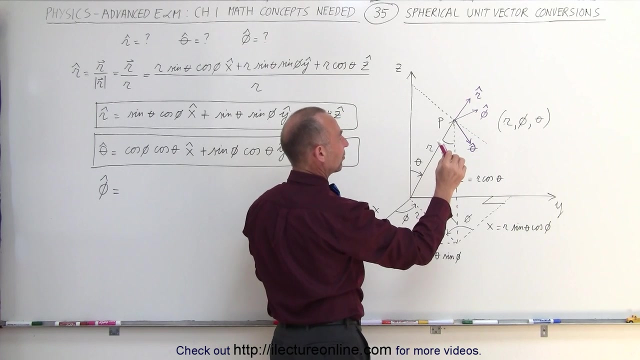 and the angle phi is equal to zero, then the phi unit vector points into the y direction. so you can see that, that when the angle is zero. let me start all over that again, okay, okay. so, looking over here, this represents the the phi unit vector and this represents my z-axis, right. 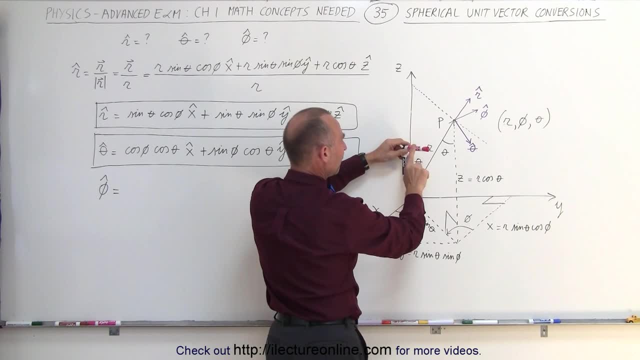 if the phi angle is zero, then the phi unit vector points in the direction, in the y direction, because it's a 90 degree direction between the theta unit vector and the phi unit vector. so when phi is equal to zero, my phi unit vector points into the y direction, which means there's 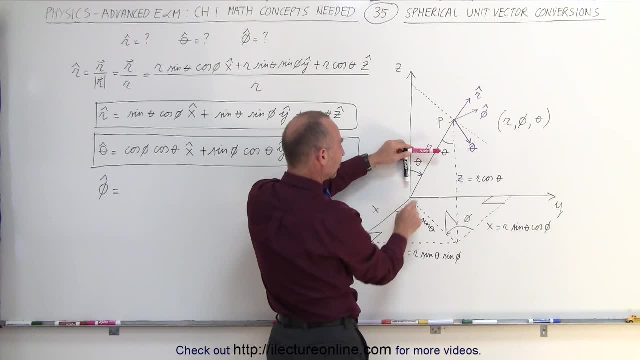 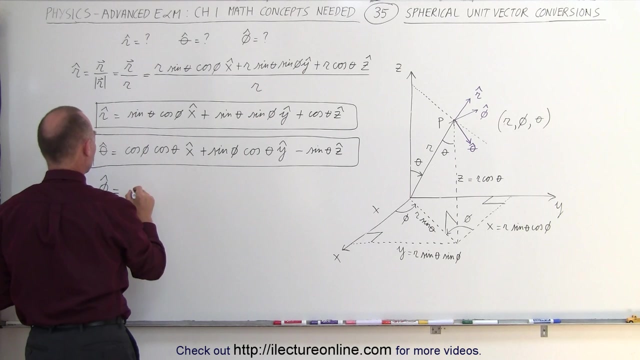 zero component in the x direction. when the angle is 90 degrees, the phi unit vector points in the negative x direction. So it's maximum at 90 degrees, it's zero at zero degrees. that is the sine. but since it's pointing in opposite direction, it would be the negative sine. So for the x,